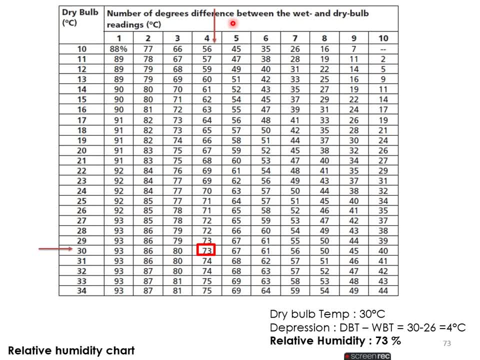 So for example, we have seen in the earlier charts, like the dry bulb temperature is always higher and we know the wet bulb temperature is always lower. So for example, if there is a dry bulb temperature of 30 and the wet bulb temperature is almost minus 26.. So the depression or the difference is going to be 4 degree Celsius. So that's given here. So if you mark from here to here and mark from here to here, you will see, you will get a relative humidity which is about 73 percentage. 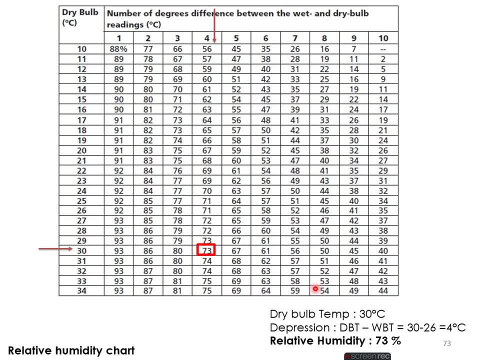 Which means that it is, it is having a lot of moisture content in the air. So that's why the humidity levels are a little bit higher. So if the relative humidity is between, it is considered best. if it's between almost like 40 to not 40, it is considered best if it is between 50 to 60 percentage, or maybe 45 to 60 percentage. So it's the medium where the human can feel very comfortable. neither it is too too moist or neither it is too dry, etc. So this is the way 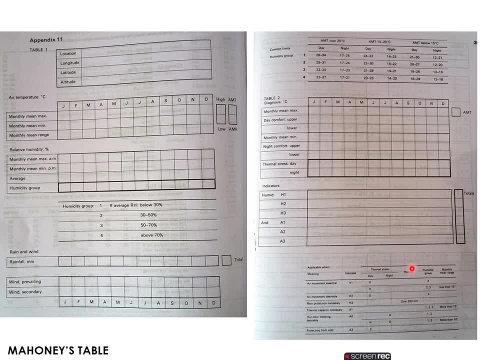 we can find out the relative humidity. The next one is, as I told you, like it is a very interesting chart, It's called Mahoney's table, So there is a set of tables which we have to fill up all these items. So you will get, after filling all these things, we will get certain recommendations. So according to the recommendations, you can know what type of design can be incorporated or what type of design can be executed for the certain climatic locations, for the certain climatic locations. So the 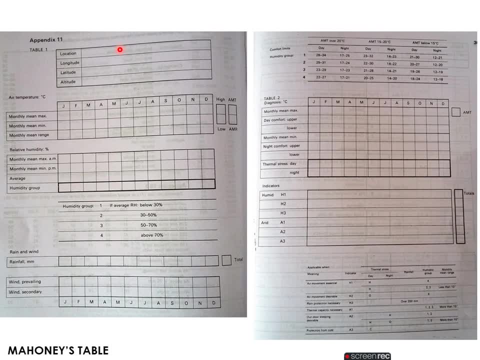 basic data has to be collected from your internet or maybe from your authentic source of books, etc. So, for example, you get the locations- latitude, longitude, altitude, etc. You will be able to get this monthly mean maximum and monthly mean minimum, which is the day and. 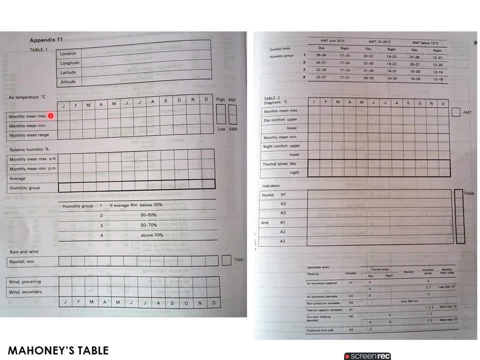 nighttime temperatures. So you have to be very clear: maximum is daytime and nighttime is minimum. So you get an average of this. So we know how to calculate all this. Then you will get a high and low. you will get amt, which is annual mean temperature. 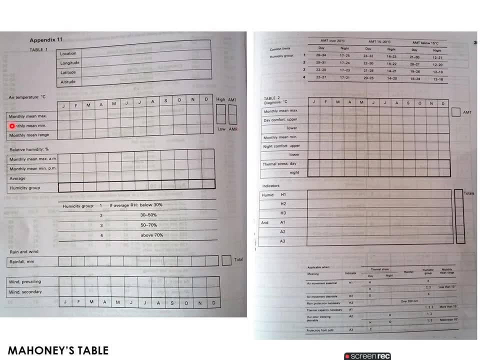 amr, which is annual mean range. so this table is actually in the book called manual of tropical housing. uh, the author is oh coins burger. so you can go through the book and if you see the book there will be certain steps which they have given and explained you how to do the calculations. so 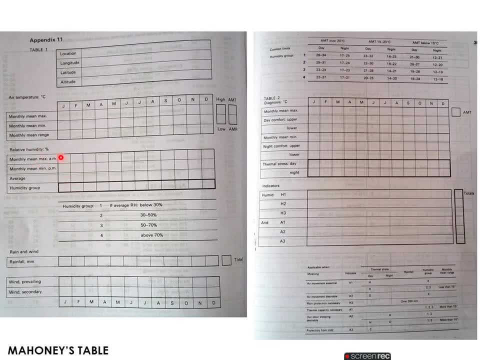 you will get the few data about related humidity. of course, sometimes you will not get this am and pm, so you can get an average of relative humidity for all all around the here. so you can get that. so, because of by finding all these things you will get into, you know what type of group it is. 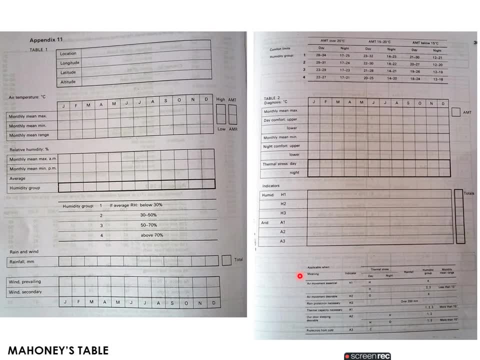 falling under. so you will also get data about rainfall, the wind, etc. and with all these data you will go to the table number two. you will fill up this table number two and with all these data you will get this thermal stress day and night by. by knowing all this thermostats, day and night, you 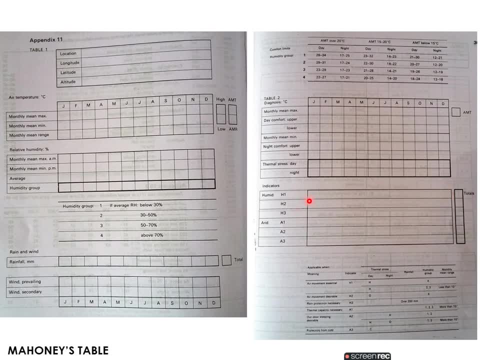 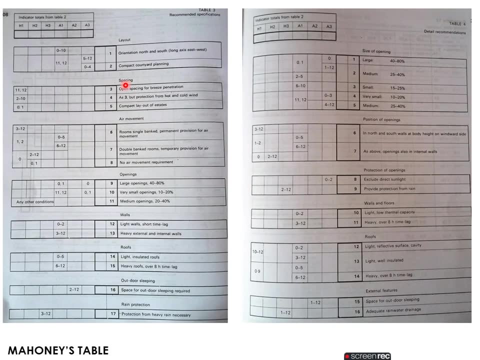 will get the data here and you will actually tick here, like how many uh ticks are going to come. you can see this data. so, according to this chart- okay, so that, anyway, i'll explain you about this- the next forthcoming charts: uh, then you will get the next table, which is, uh, going to give you a lot. 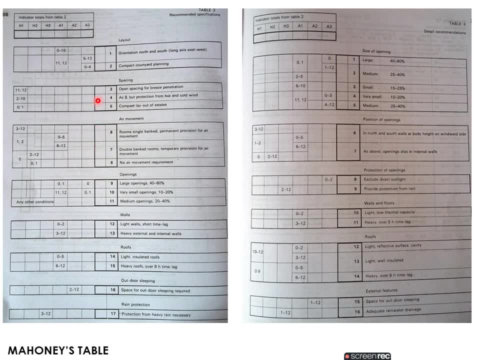 of recommendations so there is every every table. there is going to be one tick which is going to give you a lot of recommendations of design, so it's maybe like it will. it will recommend you a layout like compact courtyard planning if it's a spacing. so it will recommend you like what is the. 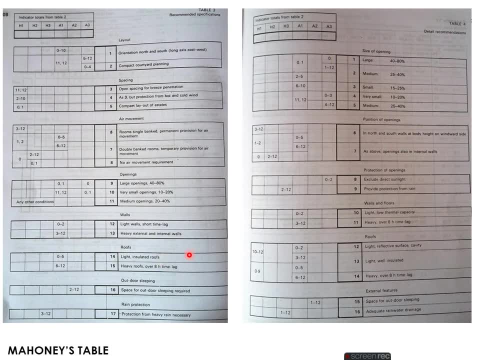 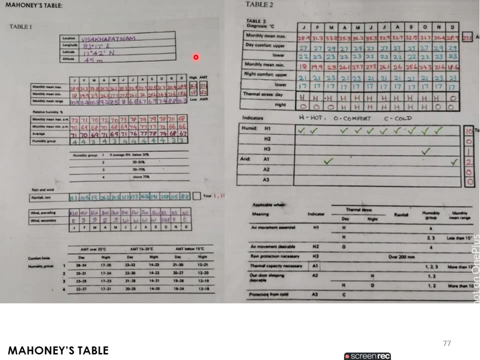 compact layout of spaces, air movement, openings, walls, roofs, outdoor sleeping, rain protection, etc. so this is again, uh, and a little bit of intricate or in-depth recommendations which you which will be recommending. so, if you see, this is an example of our student who has done the mahoney's table, so you can see she has done it for vishaga partner. 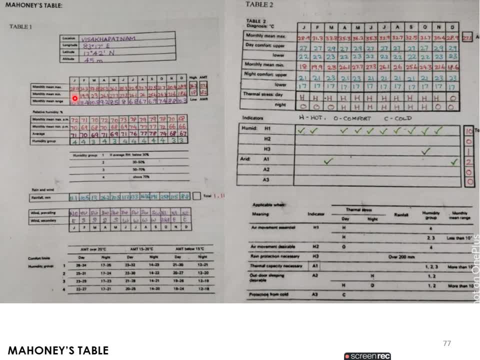 so you can see her. so she has done this monthly maximum and minimum. of course she has found out the range, so it's divided by two and again you have high and low amt, your fire e. she has found out the relative humidity. so if the relative humidity falls between 50 to 70, percentage it. 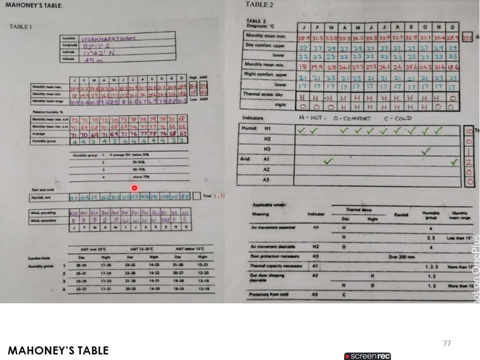 comes under the group number three, so 69. so it comes under group number three. if it falls above 70 percentage, it comes under group number four. so it is actually written as four. so she has written the data of rainfall, the wind prevailing, etc. now, if you see again, uh, the annual mean temperature if it's over 20 degree celsius. 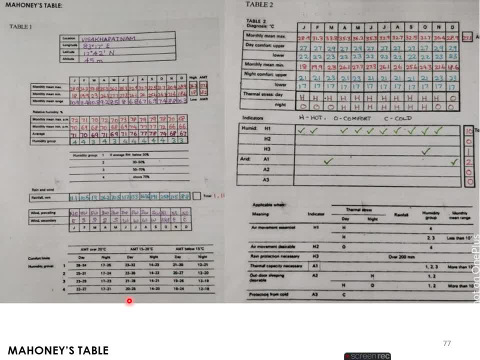 so we have to consider this chart. if it's uh from 15 to 20 d, since it have, this has to be considered. and if it's below the 15 degree celsius, this has to be considered. so if you see, uh, basically the amt, almost 27 point, something like that, so 27.1, so, which is actually more than 20 degrees. 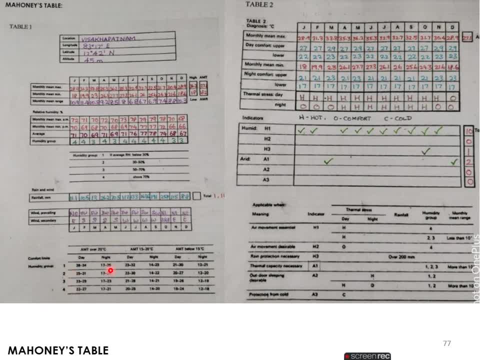 so what you'll do is you will take this, uh, this portion of the chart, okay, so now you will try to incorporate this here. for example, if it's january, so monthly mean maximum is taken from here, from 28.9. it's already there. the monthly mean minimum is taken from here, so 18, you will come here, okay. 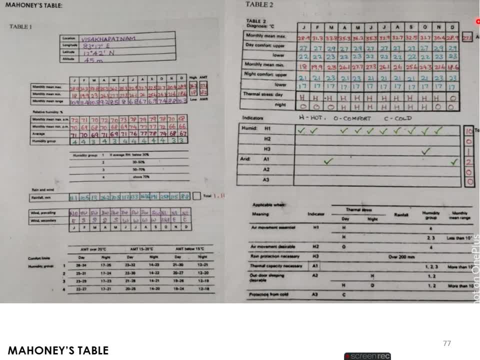 now what will happen is you will find these two results. now it's it's giving you amt is more than 27.1. so what will happen is you will take this chart, okay. so we have to see what group it is falling. so, for example, it's falling under group number four, so january is falling under group. 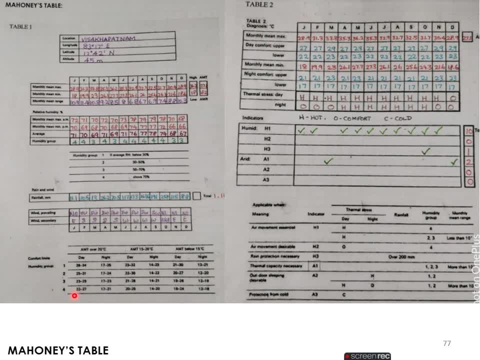 number four. so if it's falling under group number four, we have to see what is happening in group number four. it says daytime, it is going to be comfort levels, or it's called thermal stress, which is 22 to 27. so it's given here: the lower is 22 and it's the upper is 27 and during the 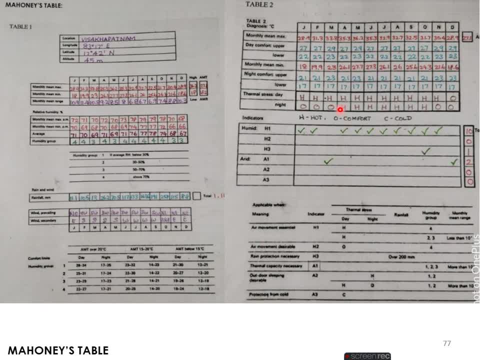 night time. it is all already done. it is 17 to 21, so again it is put here: 17 to 21, so it is already 20 to 21, etc. so now, uh, by comparing all these charts, okay, now you will find out like what which. 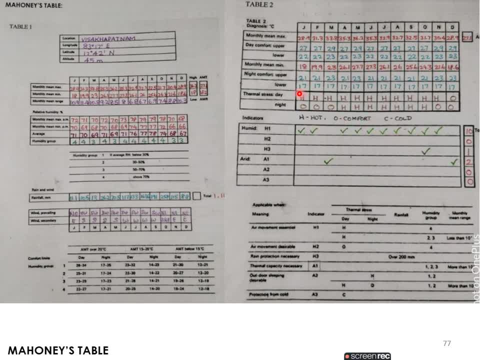 is hot, which is comfortable and which is called whether the daytime is comfortable. so if, uh, this minimum is falling under this or it's it's falling, uh, above this, then then you will get hot, or something like that. so you will know about this, uh, in your next sessions of doing it. so you will now. 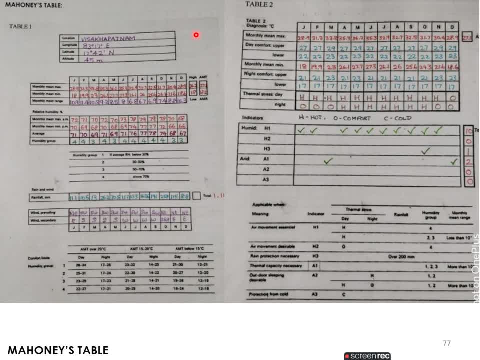 find out which is hard, which is comfortable, which is called since vishagapetnam. of course it's a humid place, so you can see like it's. most of the things are thick here on the top level. so it says air movement is very essential here. so this is the way you have to start filling your mahoney's table. 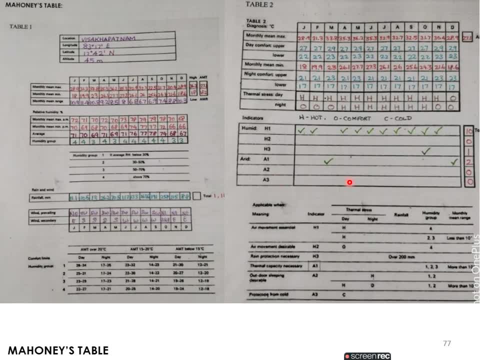 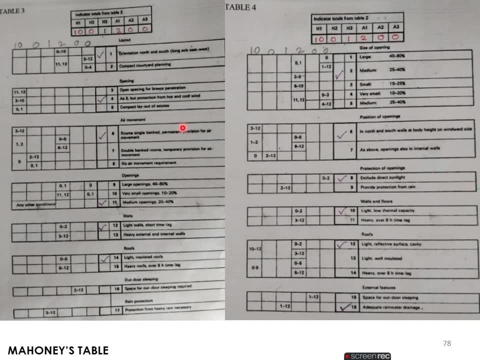 so after this, again, you will get- uh, we get all the sticks, so you will. you will find out ten zero one, two double zeros there. okay, you can find out all this. so what will happen is: so, you, you will find out all this and you write it here, so all this can be returned here and uh, this will find under. 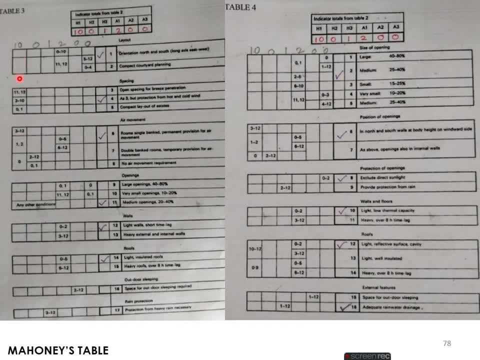 some categories, so it will fall under some category. for example, 10 is here, so this is falling under the second category, which is two to ten. so it says: uh, protection of uh hot and cold wind. so maybe it is, it is. it is like that in winter also, so maybe it. 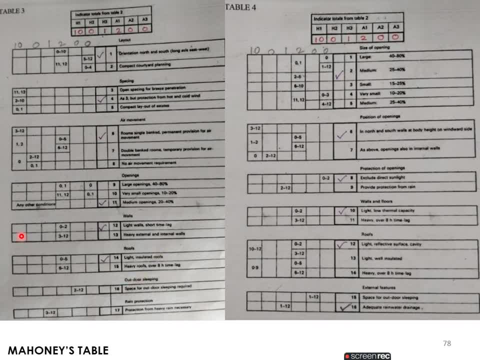 is protected. now protection is needed, so maybe what will happen is: uh again, you can see this chart two. two is falling under this category, so in the walls, zero to two. so light walls. uh, with short time lag is better, so you can write it as light watch, which is better, okay. 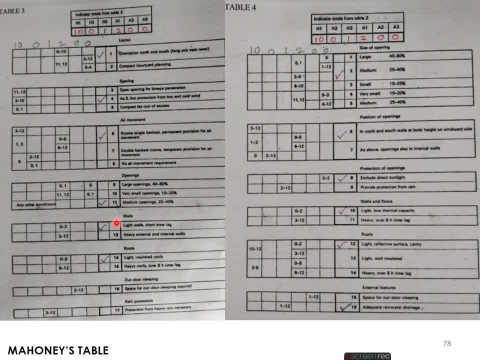 it's warm, humid place, so maybe it is already having humidity. so light walls are recommended so that the heat transfer can be left out easily in the evening, because maybe the breeze is more so like that. so you, you will come into some certain design conclusions or design ideas by doing the mahoney's chart. this was the first basic chart which was 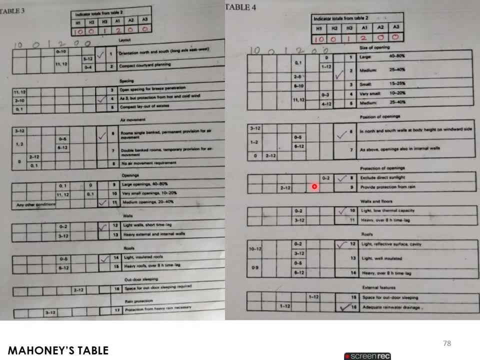 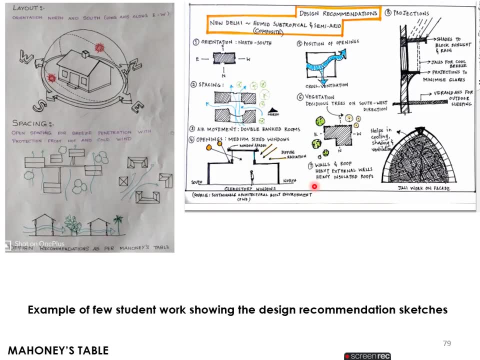 initiated by mahoney or which was done by mahoney, so that people can use it to get a clear idea of how you can proceed with design ideas. thank you, and a few more. uh, whatever the recommendations which are here is actually done as sketches by our students. so generally, again, two students works are there, so 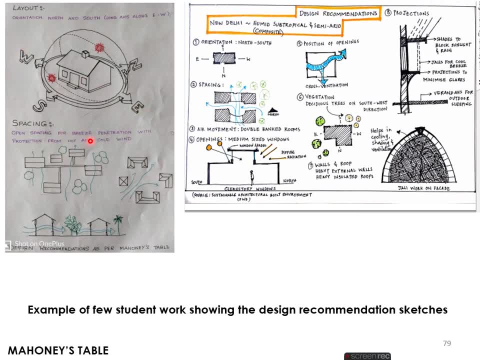 again one is like what is the type of orientation which you have to do? what is the type of spacing which you have to do? and again another student's work for new delhi she has done, like what is the position of opening, what is the type of spacing which is recommended? so whatever is done in the 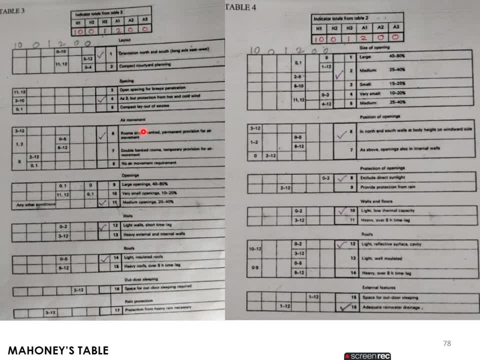 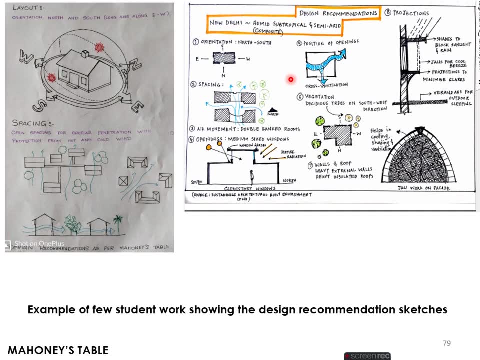 previous uh charts to layout spacing armament. all these are converted as sketches because an architect can better deliver items in a through sketching attachment and this type ofモ ҨҨゕ ғе –2 is designed to highlight never mean. 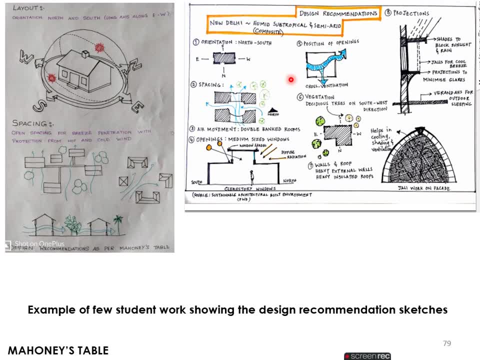 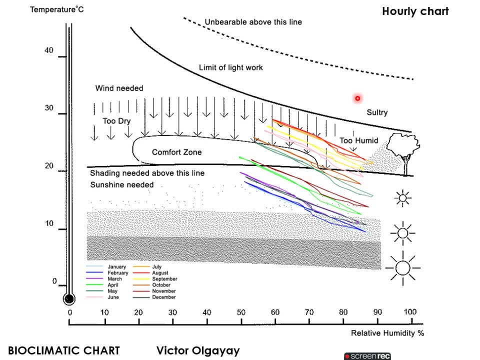 in any form of máquinette in a scenario. We generally know the comfort zone by means of little bit of subjective responses, like we know that people are very comfortable at a certain degree of about 20 to 25 degree Celsius. So this comfort zone is actually marked by means of subjective responses and of course we know beyond 27 degrees or beyond 28 degrees it's little difficult for the people to feel thermally comfortable, and below 20 degrees they feel very cold. 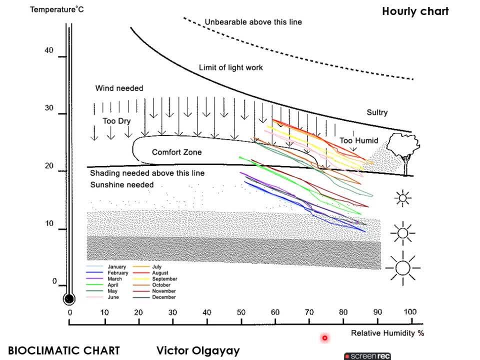 Now in a bioclimatic chart. what happens is we get general data about temperature every day and about relative humidity also every day and every hour. So what happens? you are supposed to plot the points every hour. So, for example, by today at 10 o'clock to 11 o'clock, if the temperature is about 23 degree Celsius, so maybe it is like 23 degree Celsius here, and if you imagine that the relative humidity is going to be about 23 degrees Celsius. 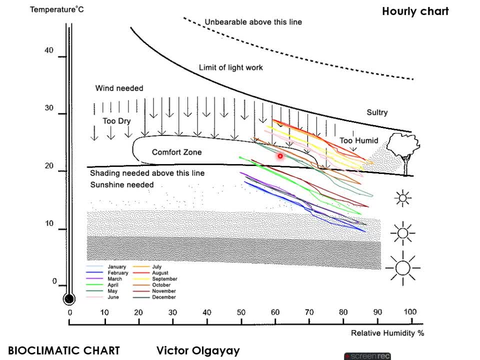 So we are going to be a little bit higher. So maybe like 63 percentage, So maybe like it is 63 percentage. So at morning 10 o'clock it is very comfortable because it's falling under the comfortable zone. So maybe at 3 o'clock during the afternoon. So maybe the temperature has raised to 32 degree Celsius, So it would be somewhere here, 32 degree Celsius and the relative humidity would be very less. So maybe the relative humidity is almost like 40 degree Celsius or 40 percentage. So your points will fall here. 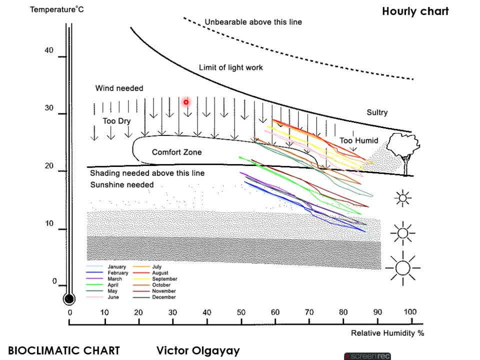 So what happens is here. Here, the recommendation generally given is the wind is supposed to be needed because when you have a relative humidity lesser, So if you try to induce wind or if you try to provide a natural ventilation or an artificial ventilation, Okay, So you will be bringing the comfort inside, So you will. you will come and sit inside the comfortable zone, Okay. So that's why the wind is needed. as you go, The temperature is higher and the relative humidity is lower. Again, if you come to night, Okay, for example, if you are in a little bit. 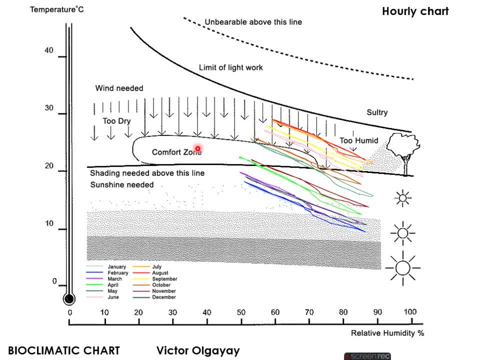 colder region. Okay, So during your night So maybe maybe it is like only 15 degree Celsius or something like 18 degree Celsius, and relative humidity is little higher, because it goes to 80 percentage during the night, because the moisture becomes higher. So again it is not falling under the comfort zone. So people need a little bit of warmth, or maybe they need sunshine, or maybe they need a little bit of heat. So maybe by in the night you cannot bring in sunshine. So what happens is we try to give 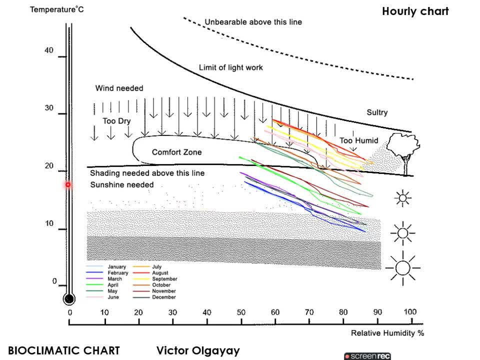 heaters etc. Fine During the daytime. if it's a very cold zone, for example if you have about 18 degree Celsius and again the relative humidity is almost 60 percentage, Okay, So what happens is the sun's radiation is needed little more inside the building to make you very comfortable. So we try to give you a little bit of glass, facades etc. So that you bring in a lot of heat inside the building. in a colder zone, in a colder zone. So again, here it's the limit of work, or it's too sultry. So points for. 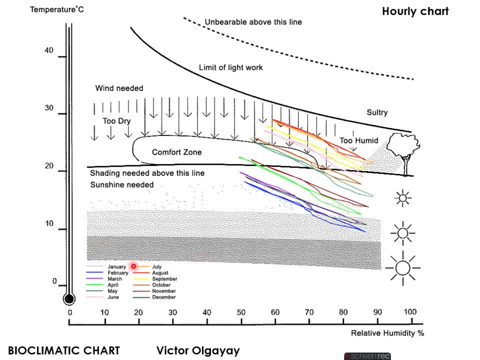 falling there will be very high. So now you can see some few charts, like January. so the points falling from day and night, day and night, day and night. So you can see the points will vary day and night for every hour. So we have about 8000, 760 hours. So we have to plot about 8000, 7, 60 hours of points so that we can understand an average value of how much. how much of points are falling under the comfortable zone. So 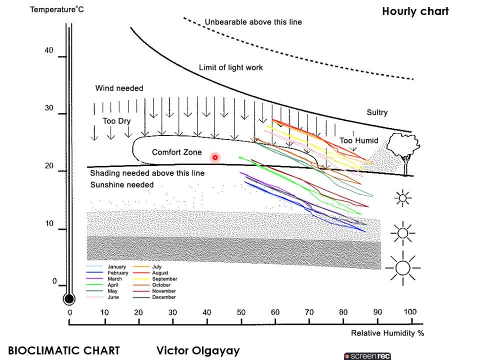 So maybe like 3000 hearts or 4000 hearts, So people are feeling very comfortable. So you can find out like so in this climatic zone, so people can feel comfortable of about dash hearts. So maybe it can be done month wise also So we can understand in which month they are feeling very comfortable. 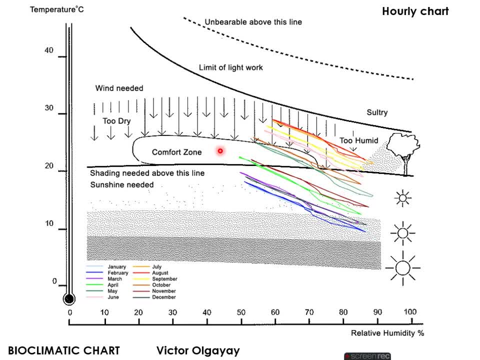 So maybe in January, maybe in February, maybe in September, August, etc. Again, the months are divided into summer, winter, autumn and spring, So we can understand by means of months. So this is one of the charts which explains you or which gives you the data of about the comfort zone. 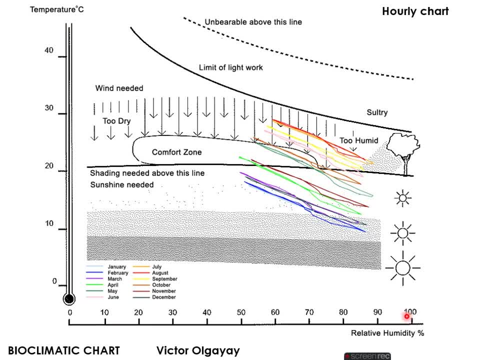 Now, these values which you are supposed to find out, the temperature and the relative humidity values, are available in the, in the internet or in the web, And it is actually a data which is given by imd. imd is nothing but indian meteorological department or any. 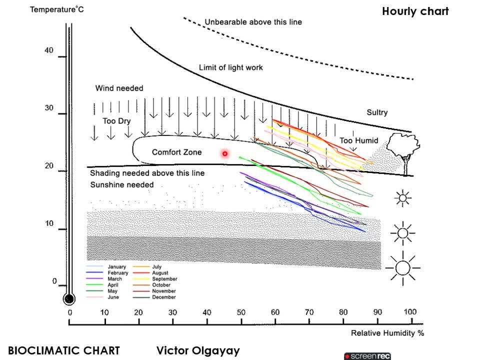 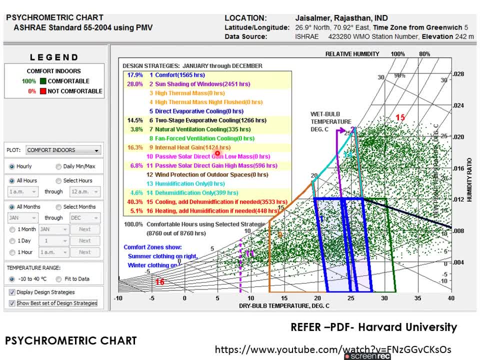 region. so this is the bioclimatic chart. so next thing is a little enhanced. so after the bioclimatic chart there was something called as a psychrometric chart, in which in the previous chart you can see the temperature was on the y-axis and the relative humidity was on the x-axis. now you see the next. 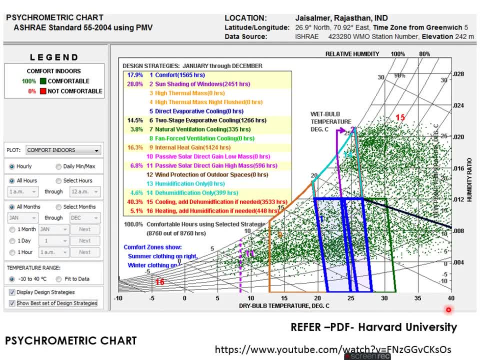 chart. the x-axis will have the dry bulb temperature and the y-axis is going to have the absolute humidity and there is a small curved line- okay, it's a thin curved line- which is also called as the relative humidity. so we understand: relative humidity is the proportion of a, h by sh. that is absolute. 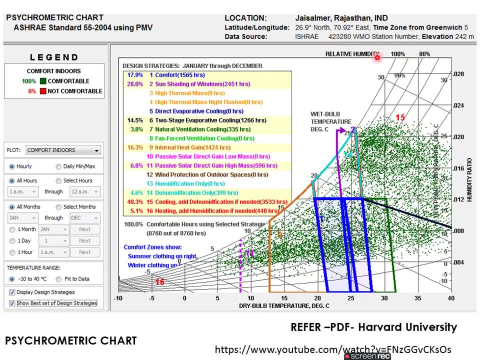 humidity divided by the saturation humidity, which is given in the percentage, so 100 percent, 80 percent, etc. so these curved lines are called as the relative humidity lines and there's a little bit of slanting lines which is also called as the wet bulb temperature, which is also called as the 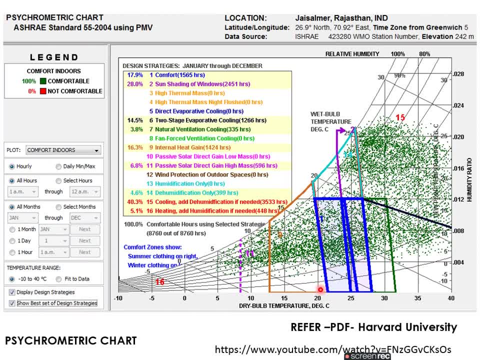 wet bulb temperature. so these lines which are projecting out from the x-axis is called as the dry bulb temperature, and these were vertical. these horizontal lines are called as the absolute humidity, so this slanting lines are called as the relative humidity. so 190, 80 and we have 70, 60, 50, 40, 30, 20 and 10 degrees. it's very low now. 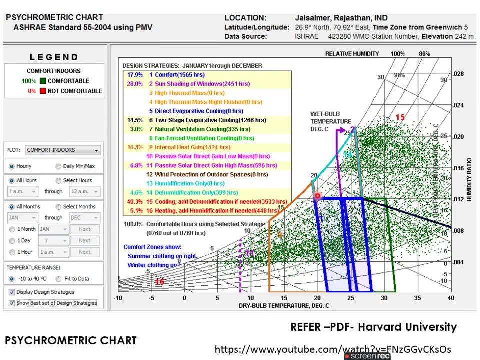 this blue color line is called as the comfort zone and these green points are called as the hours. that is 8760 hertz. now this is marked in j salmer. so it's a small typical example. actually, we can go through this software. we are going to explain you another video regarding the software itself. 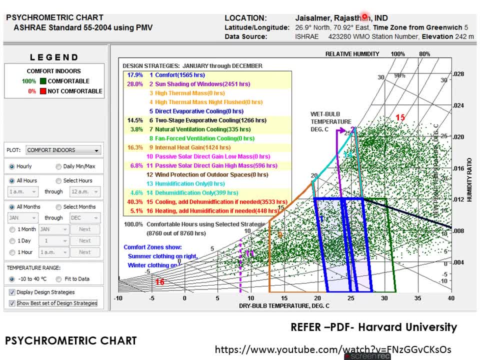 so if you see the a lot of points in j salmer, it's a very hot and dry region so you can know like it's going beyond 40 degrees celsius, so the temperature is very high. the humidity levels are a little lower. also in j salmer in few seasons, that is maybe in january or february, the temperature 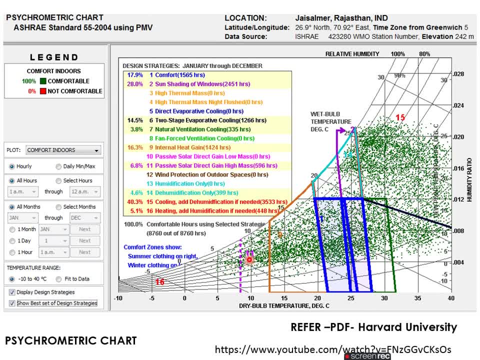 is little lesser or very less, also to 10 degree celsius, and the humidity levels are also very high. so, since it's a desert region, so you will have both the types of humidity that you have in the desert region and also the types of, uh, what you call the variations of climate, so there will be a 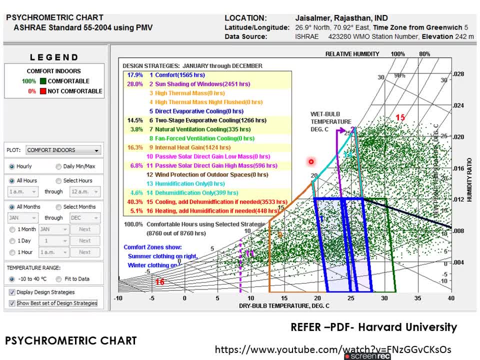 lot of diurnal variations, which means the daytime can be little hotter and the night time can be little lower. this software- now the psychrometric chart- was done manually. now the climate consultant software is actually giving you the psychrometric chart by means of inserting a data called epw data. 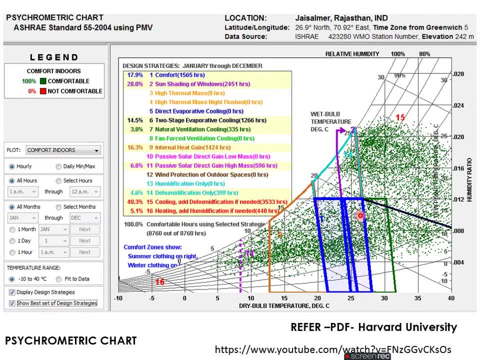 so now climate consultant is the software so we can see about climate constant later. so this software is a very good software which gives you the whole picture of the climate, Okay, And it also gives you the types of strategies which can be incorporated to what you call maximize the, what you call the thermal comfort. Okay, So that is the way it is trying to do it, So we can see about it. So this is the region of comfort zone. So if you have this green color, for example, natural ventilation, So if you use like almost a 3.8 percentage of natural ventilation, I can- you can bring in more comfort. So this is called internal heat gain. That means it's cold. 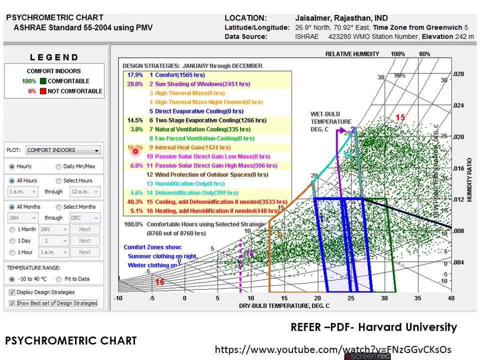 Okay. So if you want to bring in a little bit of almost like 16 percentage of internal heat gain, if you put something like: if you use a lot of what you call thick walls or etc. Or if you use a little bit of fireplaces, etc. You can gain heat, or maybe by means of using glass windows. So this will actually give you more comfort. So this is the way we are going to see the psychrometric chart in the later slides. 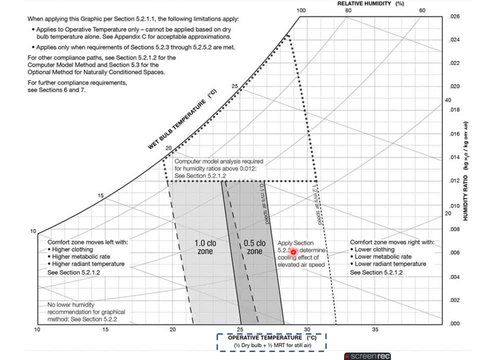 So again, there is something called as a straight standards, American Society for heating, cooling and depravation, And this actually standards is actually giving you a standard of comfort zone. So this is the standard of comfort zone, which starts from 23 degrees to almost like 27 degrees Celsius. So this comfort zone varies. if it's like 1.0. It also gives you the clothing level. So, as we saw, what is the metabolic rate and what is the clothing level, So it's also giving you the clothing level. So, if you are points or weather data points, if it's, 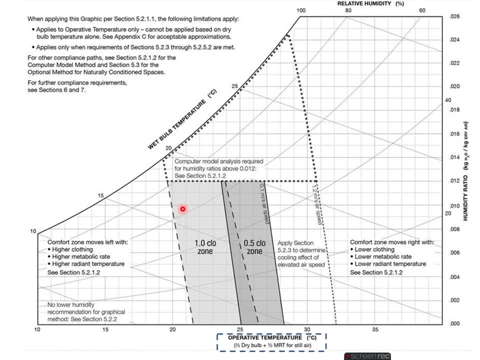 falling under this category. it means you are feeling comfortable during the winter and also in summer. So 0.5 is almost for the summer, So you are plotting level is lesser, So 1.0 is for the winter. So if your points are falling here and if you wear a suit or suit or whatever it is and you will feel comfortable, Generally it gives you operative temperature or sometimes it gives you the driver temperature also that we can see later in later sections of the slides. 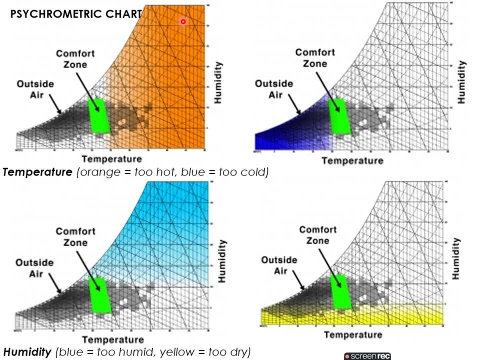 Now if you see like if it's a lot of data points are falling under your right side of the right side of the chart, it means that it's an orange color. It means the region is too hot. So if, for example, we saw about Jay Salmer and Jodhpur, etc. It's a hotter regions in India, And if your points are falling on the left side of the chart, so it means it is too cold, maybe like Shimla, maybe like Shillong, etc. So they'll fall under this. 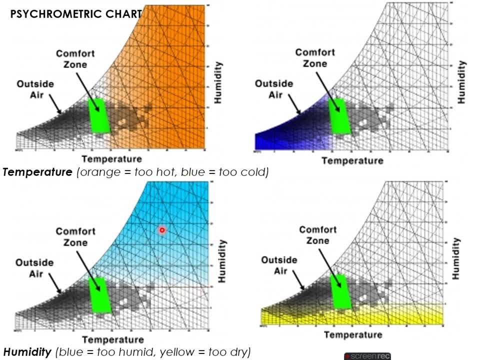 falling on the top topmost corner of the topmost right corner of the chart, it means it is humid. so maybe like chennai and a few regions like chennai, etc. so now this is the, this is the chart which is actually showing you a lot of humidity. okay, and if it's falling under, 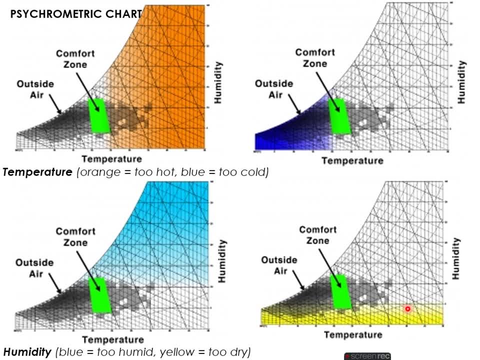 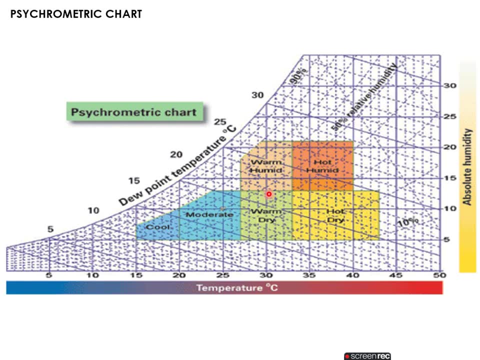 this. so, for example, yellow color if it's too dry, so maybe some desert climate. so a lot of weather data points are falling under this, so it is like two right. so you can understand. by the next chart, which is actually here, can you see if the points fall here. it's cool, it's little moderate, which? 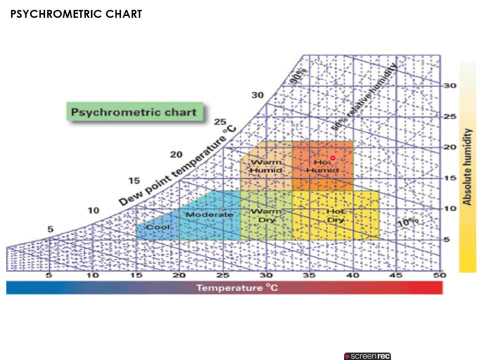 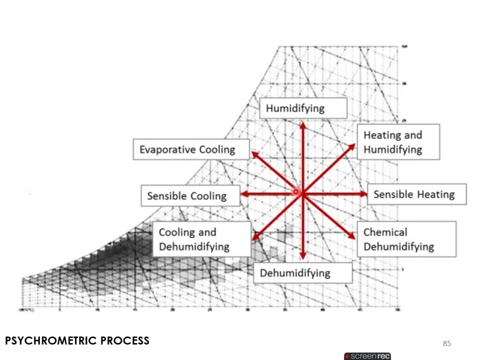 means we feel comfortable. it's warm dry, hot dry. it's hot, humid and warm, humid. so it's almost. you can see how, how, the how. the data point will actually give you the exact climatic aspects of the location so you can actually see what type of systems can be used to measure the humidity. 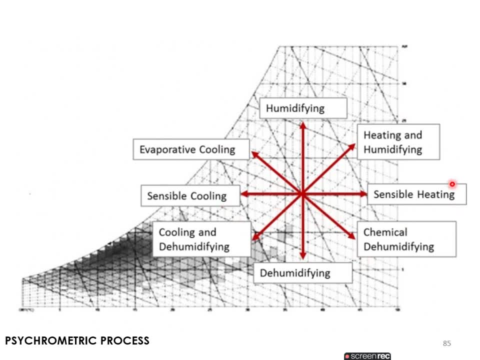 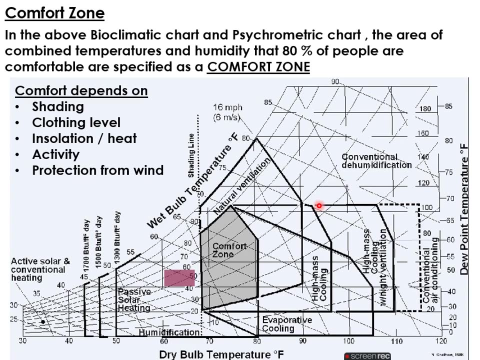 so it can be used okay with evaporative cooling, sensible cooling or sensible heating, and humidifying, dehumidifying etc. we will explain this in the later slides also. just to understand now, so you can see, comfort zone is nothing. but in a bioclimatic or in a psychometric chart, the area 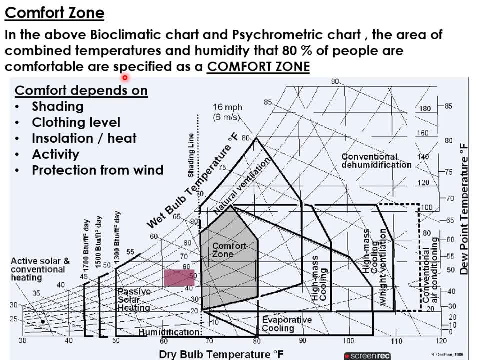 with the combined temperature of humidity in which 80 percent of the people are comfortable are specified as the comfort zone. of course there is some kind of subjective responses also. so we find out like what type of temperature and in what climate, what humidity level you feel comfortable, etc. and it depends on the shading level, the clothing level, 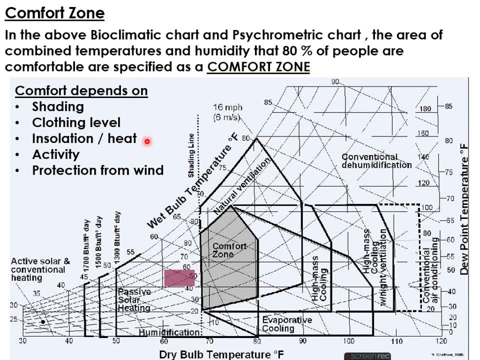 of course, the heat- what type, how much of heat is there? and the activity, and also the protection from the wind. okay, so this is the comfort zone. if you take so much of evaporative cooling, so you can bring in more comfort. if you do so much of natural ventilation, you can bring in more comfort, and so 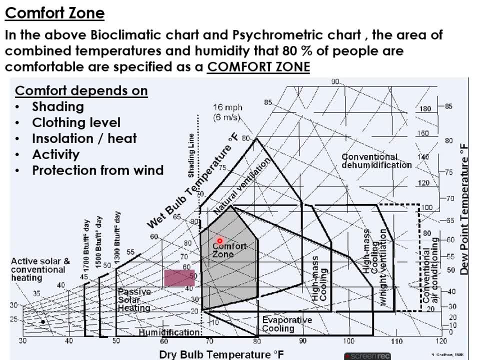 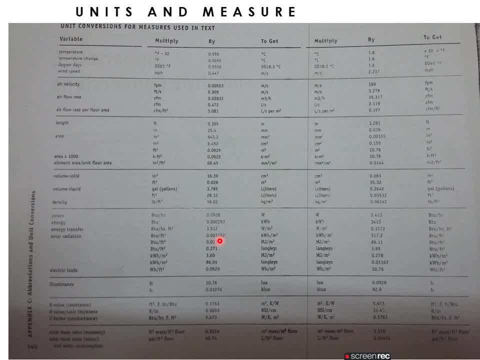 on. fine, so this is the way how a psychometric chart is going to be there and you can just understand to this level and later slides you can understand more detail about the psychometric charts. so there are a few various units and measures which you can see. 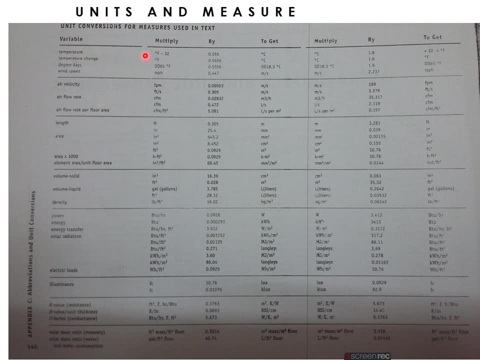 so you have to know, like if it's uh, certain things are given in fahrenheit, how to convert into degrees, certain length, areas etc. btu into some of the units, volumes, etc. so now this is out of the fundamental units. you have to just go through and find out what is the units and measure. 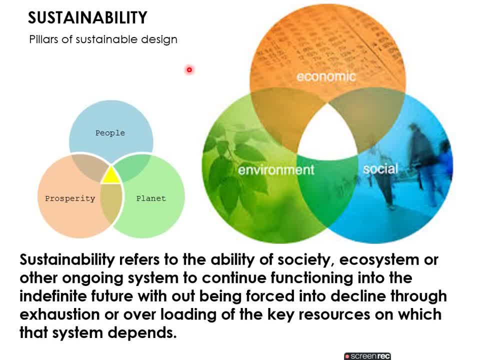 and at last now we have to really understand, like, why are we studying the subject? okay, so now we generally understand what is sustainability. generally, everybody has got a certain word. so suddenly they say, everybody today: sustainable, sustainable, sustainable, so be sustainable. so we have to really know how you can be sustainable. sustainability does not mean 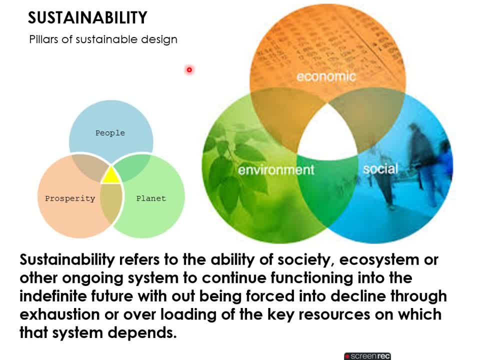 uh, just to build a green building, but it is also a way of living, so you must know how to live sustainably by means of exactly using the resources which are available with you and also giving the better environment to the next generation. so that is what is called. 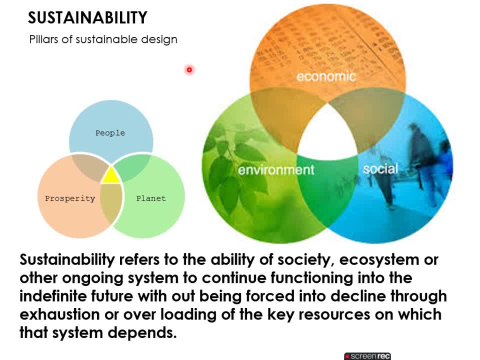 sustainability. so to sustain is is the general term. it's called a sustainability. so now there is a general, what you call the definition, which is given by the institute of architects, american institute of architects. sustainability refers to the ability of society, ecosystem or other ongoing system to continue functioning into the indefinite future. 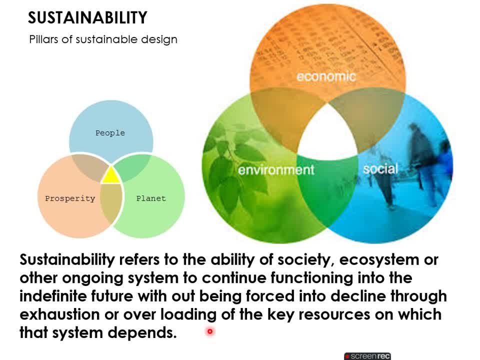 without being forced into decline through exhaustion or overloading of the key resources on which the system depends. so we have to know how the system is going on now, how to exactly use the resources which are available now and how to provide the better environment or better resources. 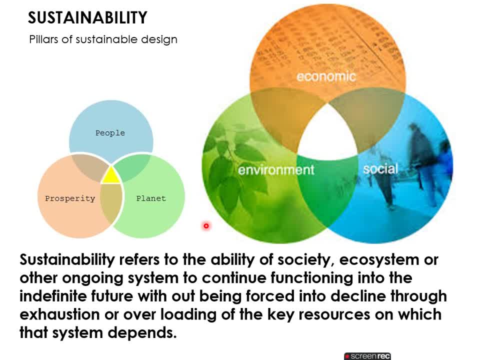 or better facilities, uh, without losing our own identity or our own energy or whatever it is for the future. okay, so now these are the key resources that we need to be able to use in the future are the three main pillars of sustainability, so we call it as the social pillar, economic pillar and 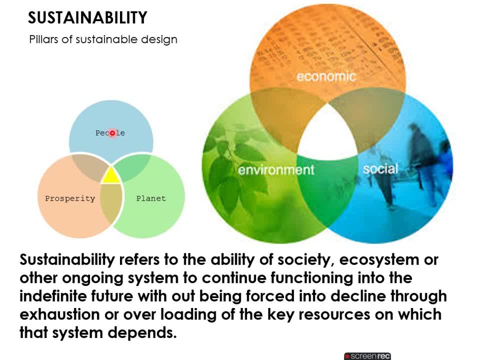 environmental pillar and it's again we call it as the three piece, which is people, prosperity and planet. so all these three have to be combined in a good proportion to get a human comfort. the yellow color is called as the human comfort, so socially. so today, if you see social, so we have a. 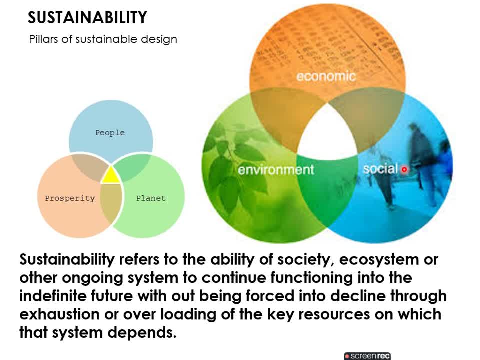 lot of social networking, but we are not social enough in terms of interacting. okay, there is a lot of interaction, but it is missing. of course, the friendship is also missing in a lot of- uh, the real, real source of friendship is actually missing in society. of course there is a lot of economy. 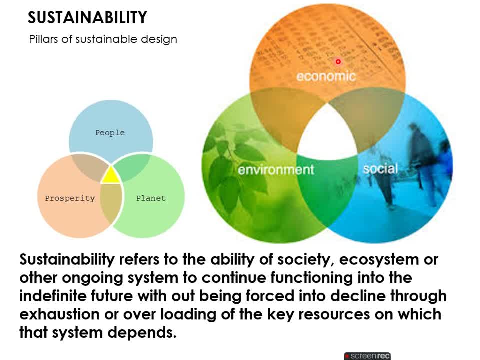 economical variations are very high. it's a very vast field which you have to discuss. so we have to combine a society and an economy to find a good well-being and we have. next thing is environment. so an architect can actually concentrate more on the environment because actually given the choice to actually change the environment, okay, an architect or a designer. 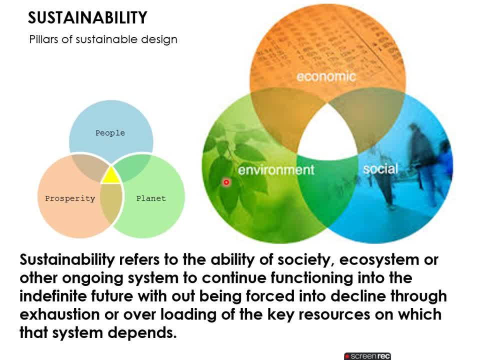 who is going to, is going to build, or who is going to design and who is going to propose something for the future- okay, for the future living. so the environment is a major aspect which is given to the architect. in such a big environment, there are small, small, small things which you can change. 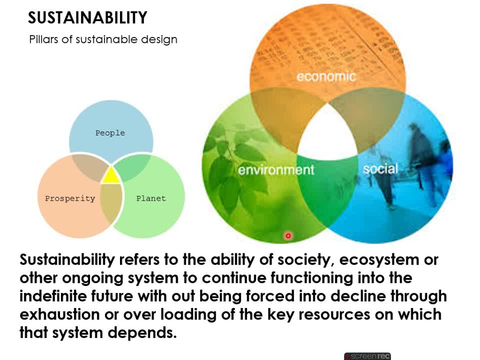 the environment is a very large world or a large arena where you can try to change smaller things as an architect or a designer and create a better future. so this climate response to architecture field is a very small field where which is more oriented towards the environment and also energy. 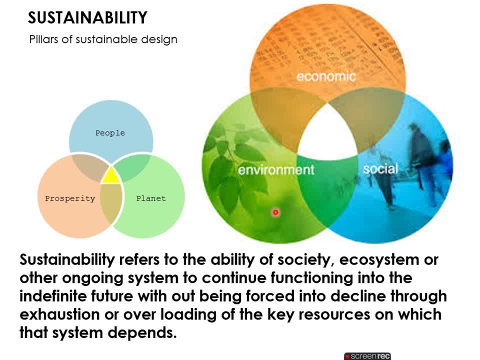 saving. so if you, if you do better and better buildings for the environment and also two buildings which are energy saving, it is going to be very economically so, due to the betterment of the environment, the society is going to give you a, a better result, or the society is going to feel. 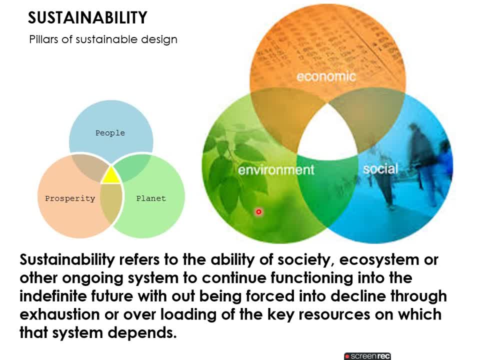 very happy. so, according to the change in the environment, the environment is going to be better. of the environment, these two are also going to integrally be better in terms of your, your sensible ways of design. so, as a sensible architect or a designer, so you try to find things like what? 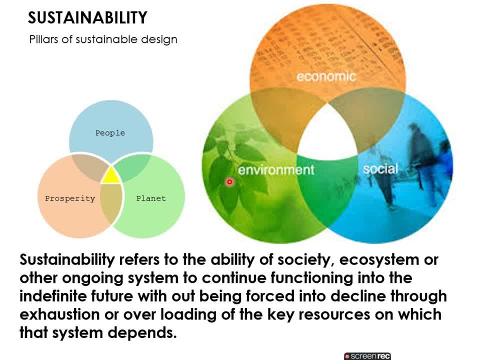 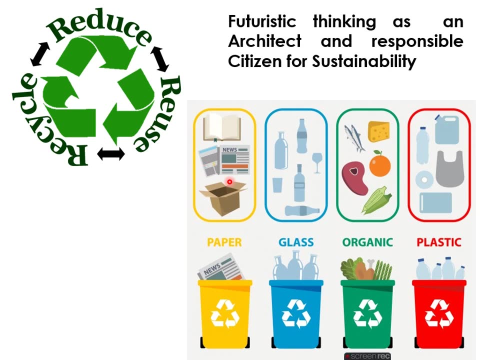 can be done in the future, or how you can give a better- uh, better- building or a better proposal to a client which is more oriented towards the sustainable future? uh, as an architect or a designer, we need to know how, how things are wasted. of course we know. in a building industry, there is. 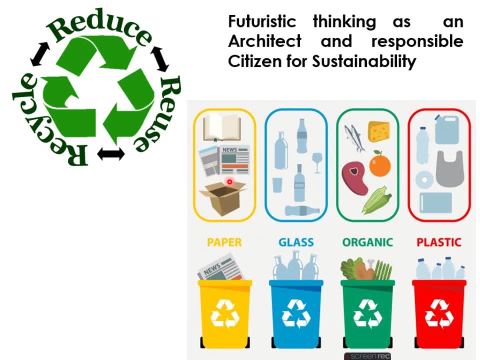 going to be a lot of waste whatever you are going to use. okay, so if you propose a lot of items which are which cannot be reused or recycled, etc. so you're going to generate a lot of waste. so waste is actually segregated into paper, glass, organic and plastic. so, as a sensible architect, you must 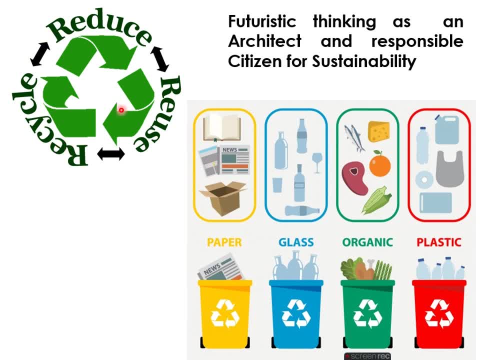 know how to reduce, how to reuse and how to recycle by means of redesign. so you have a lot of options now. okay, so a lot of new, new elements or new buildings may come up, or even an old project might come, which which can become for renovation or etc. so you can try to implement your type of 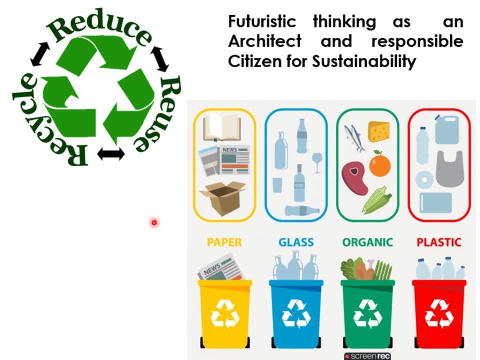 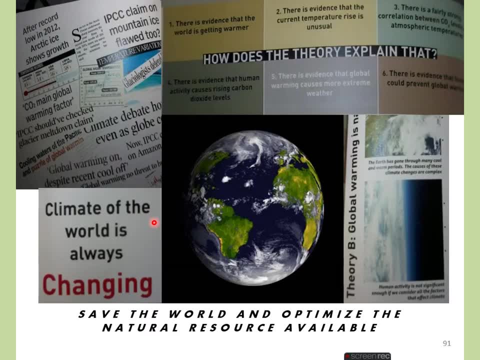 strategy of reusing certain things in a better manner. so that's how an architect must think as a responsible citizen for the future. so the climate is always changing. so be aware how the climate is changing, how you can adapt yourself to climate, first thing, and be aware that the materials are also going to change. 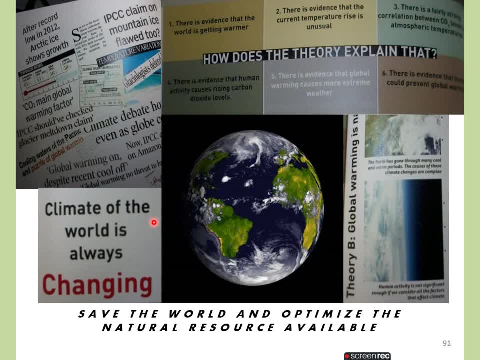 now. so be aware that there is going to be a lot, of, a lot of changes in terms of what you call the thermal thermal thermal capacity or the urban heat island effect, etc. so you have to know how you can develop yourself and give a better solution to the whole world. thank you. 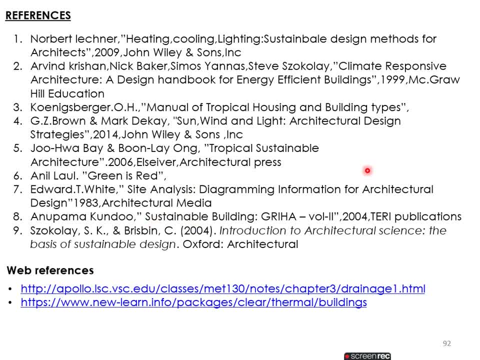 we have a lot of references, so it's a very important task, or a very important, what do you call it? it's very important to know about the books which you are supposed to study, which are very, very authentic, because these books are referred and these books are entitled, or these: 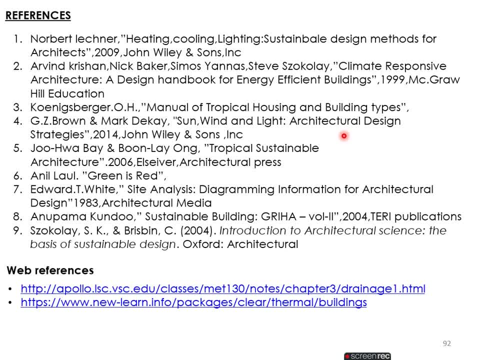 books are published by means of a lot of references by the scholars, so you can see, the first thing is heating, cooling, lighting. it's a very interesting book. this is a very indianized or maybe it's a very book which you can go through. climate responsive architecture. this is the manual manual of 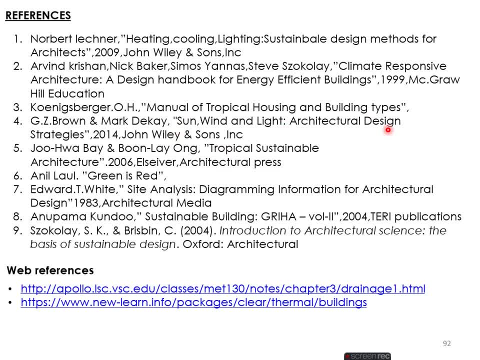 tropical housing and building types. we have sun, wind and light, which is an awarded book. okay, you can go through that. we have tropical sustainable architecture. it's a set of- uh research papers very interesting, so you can just go through this. green is red is a very nice book. who's an in anil is an. 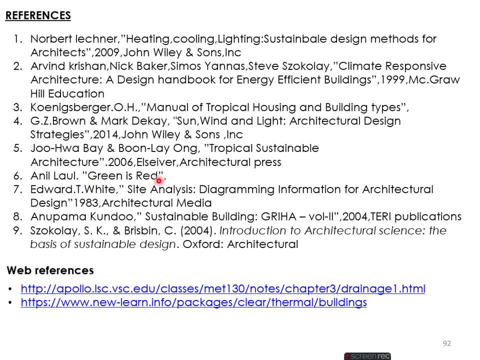 ill law is a very it's an. he's an indian architect. this is a very nice book. you have to read, or go through it, how he makes very simple buildings and he makes it very simple. and he makes it very simple, it very sustainable or makes it very climate responsive for the environment, so you can go. 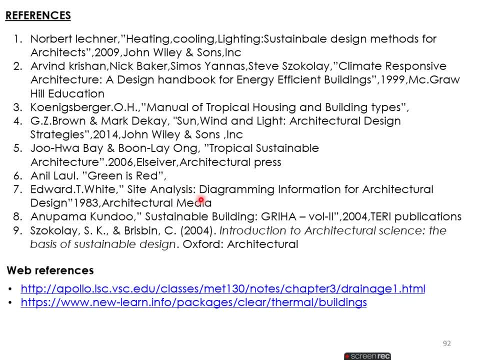 through that. of course, you can go through about site analysis, how- how an architect must perform this. this is designed by means of site analysis. we have sustainable building. we have introduction to architectural science, which is more technical. you can know about all the technical data of psychrometric chart, your heat transfer, your lighting, acoustic, etc. in this book. okay, so now. 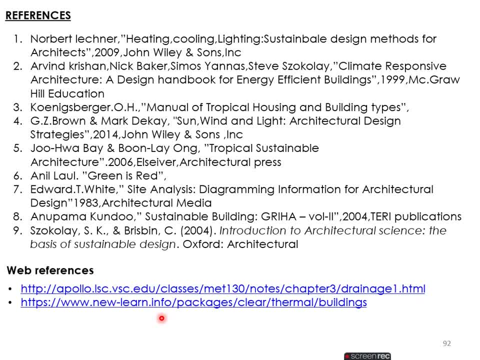 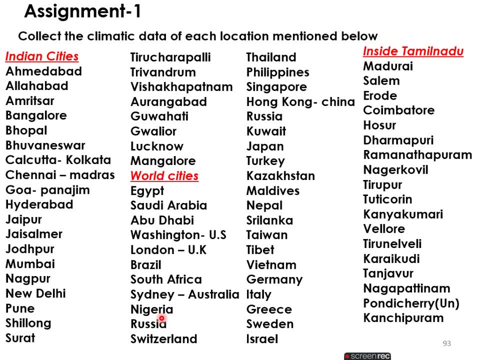 we are going to go through some of the things that we are going to talk about in this book. so first of all, we are going to talk about the microclimatic data. so microclimatic data is a data that is collected in certain points like small. i have just given only two references, but 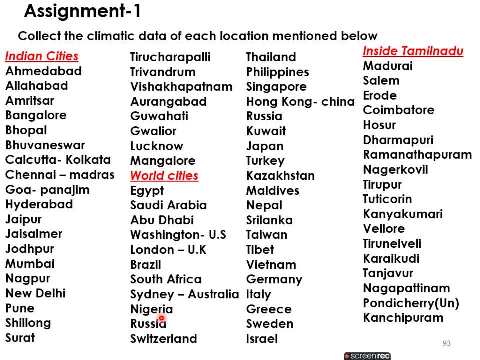 there are a lot of web pages which you can go through. okay, thank you, and we had a nice session. uh, we will be going through these assignments later, so we can just see the assignments which which you are supposed to do. so this assignment one is to climate data, which you are supposed to. 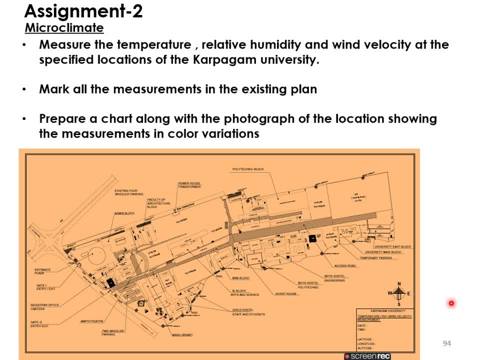 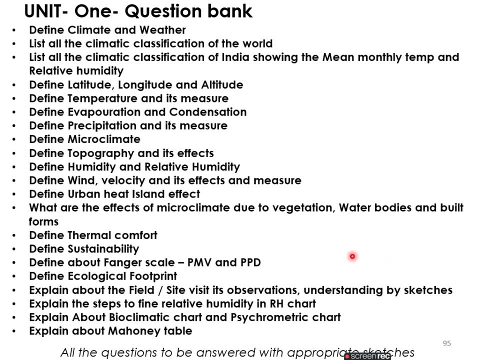 collect the climatic data which i have mentioned at inside the campus and we have question banks. you can just go through the question bags and then kindly prepare for the exam. thank you. now the unit one is completed, which is climate and thermal comfort. hope you had a better knowledge in these sessions, so we will actually 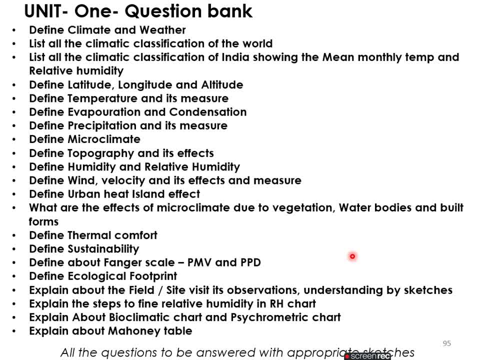 see unit number two from the next session onwards. thank you so much. all the best you. 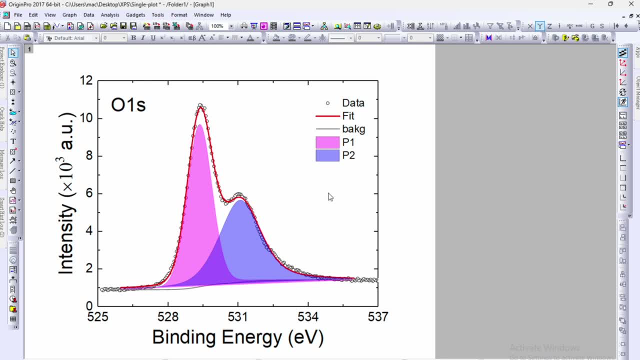 In this video I will show you how to calculate area under a curve by using origin software. So let's consider an example. This is an XPS spectra of oxygen, ONS Here. after decannulation I found there are total two peaks within one XPS spectra. Now my point is: I want to get 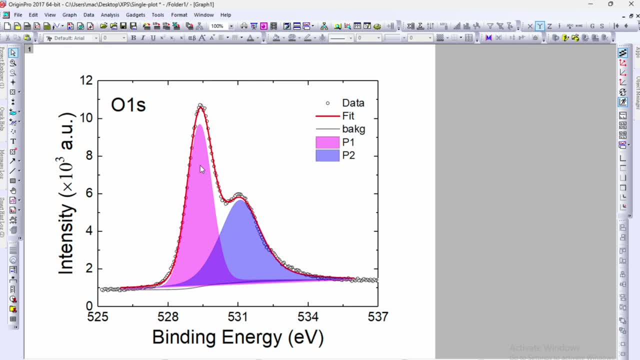 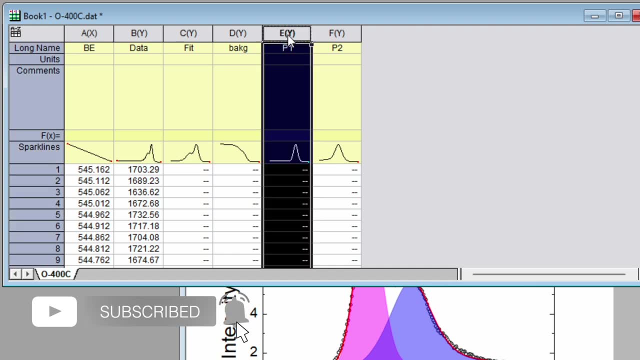 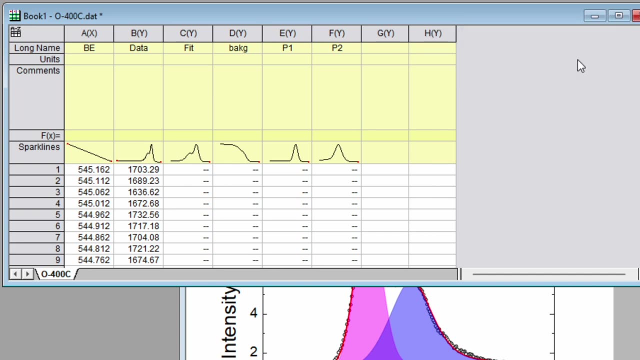 the area of each peak or the contribution coming from each peak under total oxygen XPS spectra. So how to do that one? Let's go back to the raw data. So this is a peak P1 and peak P2 after decannulation. Create two new columns Here. this is a background, So we